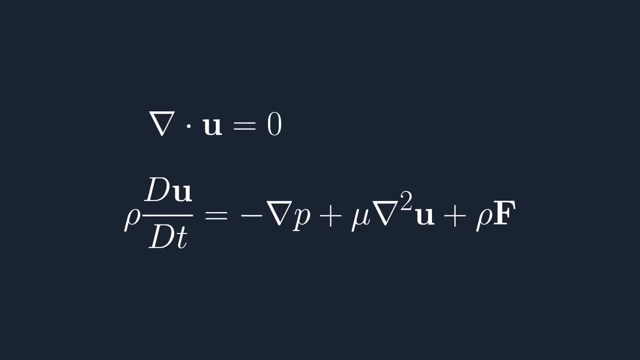 the two most well-known of which look like this: The first, shorter equations, simply states that divergence of velocity equals zero. What this means is that the velocities in neighboring areas of a fluid cannot be flowing towards each other or away from each other. 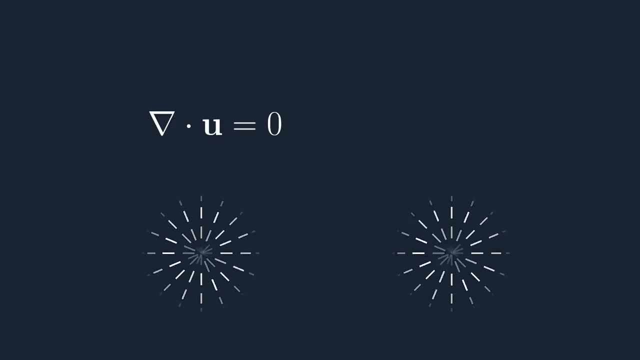 This is because that would mean that somewhere in the middle, matter would either have to be created out of nothing or disappear into nothing. Essentially, the equation makes sure that mass is conserved in the fluid. The second equation states that the acceleration of a fluid is dependent on its internal forces. 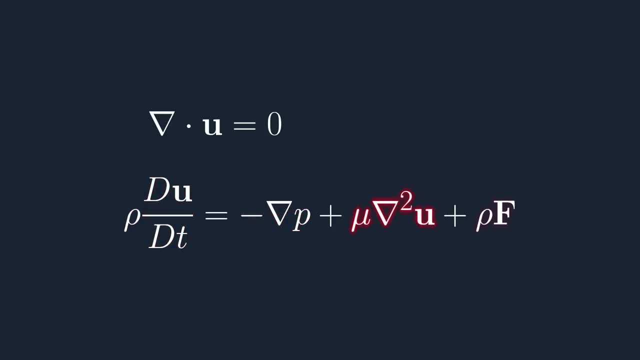 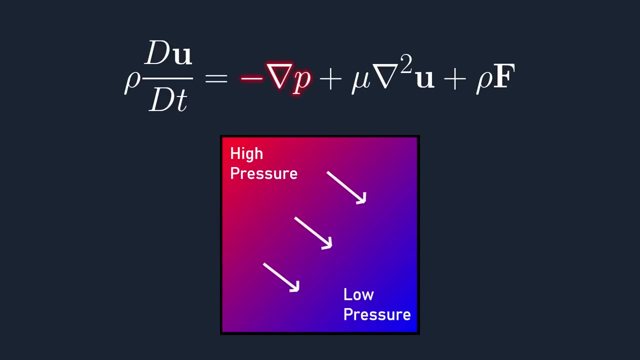 including its pressure gradient and the acceleration of the fluid. The third equation states that the acceleration of a fluid is dependent on its external forces. A fluid has a higher pressure gradient if there is a larger difference in pressure between its different areas, and the fluid will tend to flow from the high pressure area to the low pressure. 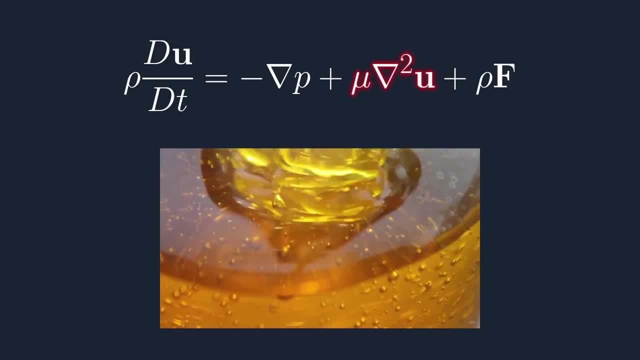 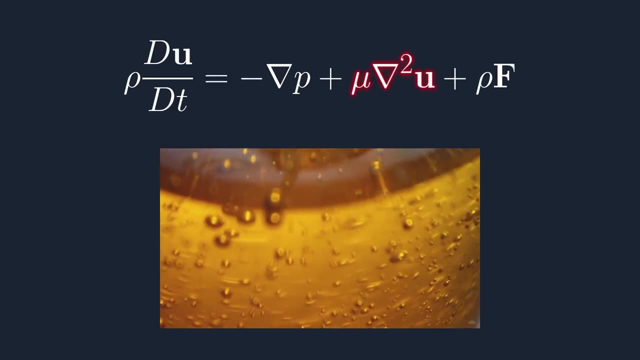 area. A higher viscosity means that there is a higher friction between the fluid's particles, and the velocity in the fluid in one spot will more easily spread out to surrounding areas. External forces just include things such as gravity and interference by objects in the fluid. 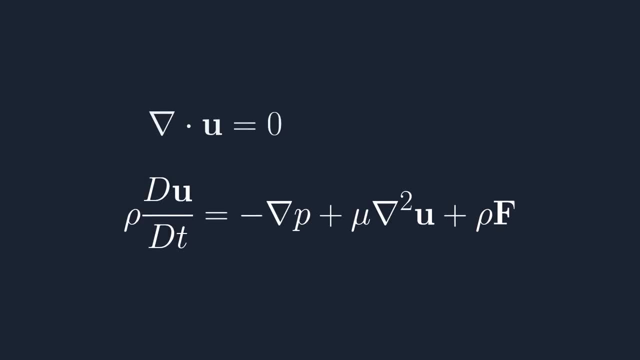 or surrounding walls. So that was a brief explanation of the Navier-Stokes equations, and you might agree that they seem to apply some fundamental laws of physics to fluids and are very important in the simulation of fluids. However, I'd like to point out that they give us the specification. 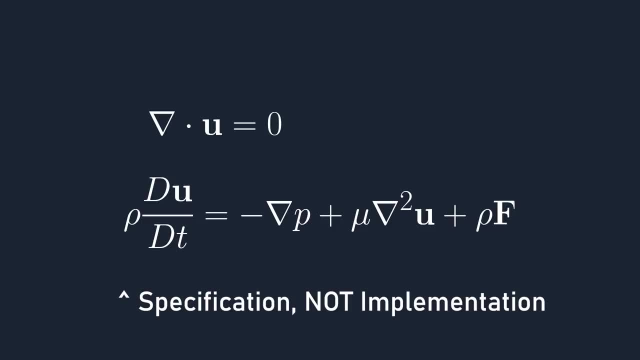 not the implementation. This means that while the equations tell us what rules our fluid simulation have to follow, they are almost useless in telling us what the simulation process actually looks like. In the rest of the video, we'll cover the actual simulation process, and, while you might, 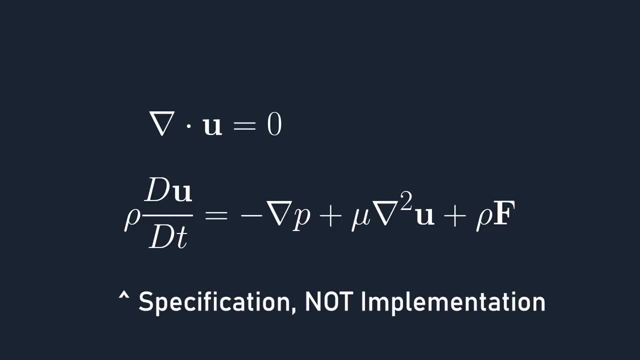 be able to see some links between the Navier-Stokes equations and the procedures which we are implementing. there are some other mathematical concepts which are much more relevant and involved. There are a few different ways to represent a fluid in a computer simulation. Namely, the simulation could either use particles which move around. 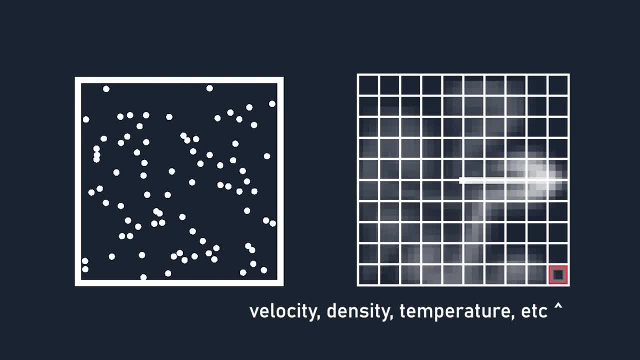 or a grid of stationary regions with attributes that represent the average of all the imaginary particles that would be in each group. This means that some fluid's particles actually represent the average of all the imaginary particles that would be in each group. So in this, in these images, I just unfolded the assembly and this was a very common clue. At the top, I can see which readers of my students preferred the fluid or if not the fluid. So now in the first example you might see that the fluid is flavorless depending on which adults are at the top here, which is not the catalyst. 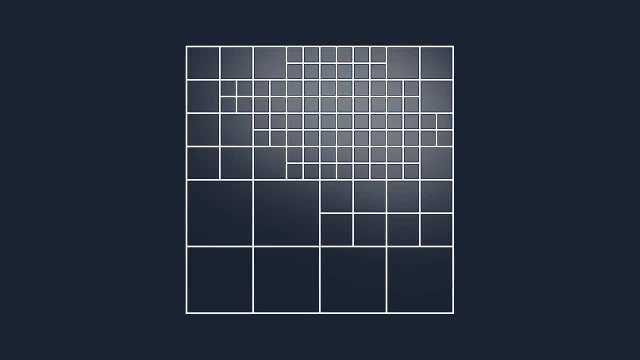 grid square. The levels of detail used to represent each area can also vary depending on the density of each area, so that computation power is used most efficiently where it is most needed. It would be impossible for this video to cover all these different methods, so we'll only 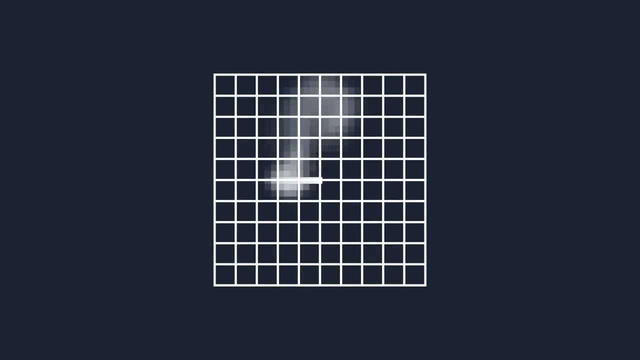 be looking at the type of implementation with a grid of square regions. without the dynamic detail allocation, All the grid squares will be the same size and stay static. Specifically, the implementation covered in this video will be going off the 2003 paper Real-Time Fluid Dynamics. 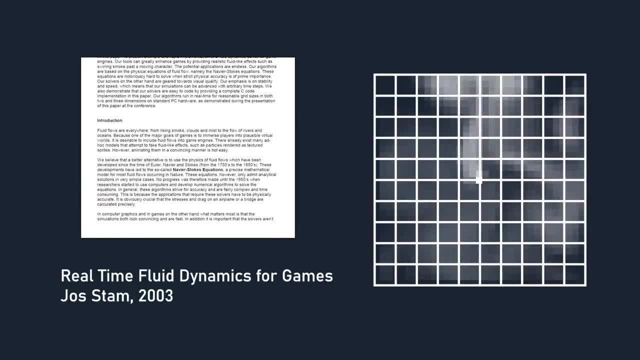 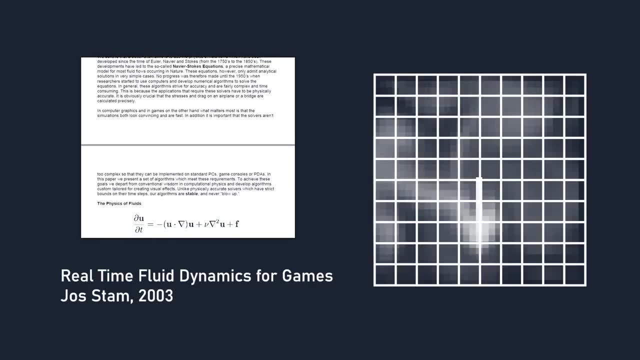 for Games, written by Yoss Stamm, which was also presented by him at the 2003 Game Developers Conference. This is a very famous paper, probably the most well-known and cited resource in the field of fluid simulation for video games. It presents a simple but effective fluid solver. 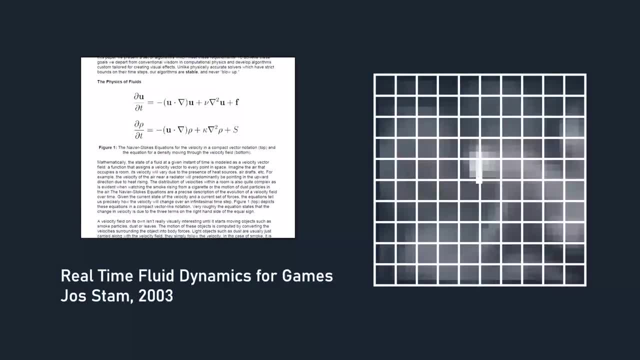 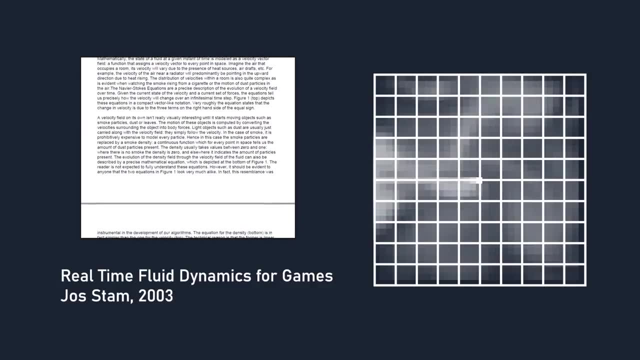 which doesn't cover every possible feature, but gets the job done and will hopefully be relatively easier for you to wrap your head around. We will also exclusively be dealing with 2D, but the principles covered in this video can certainly be extended to 3D as well. 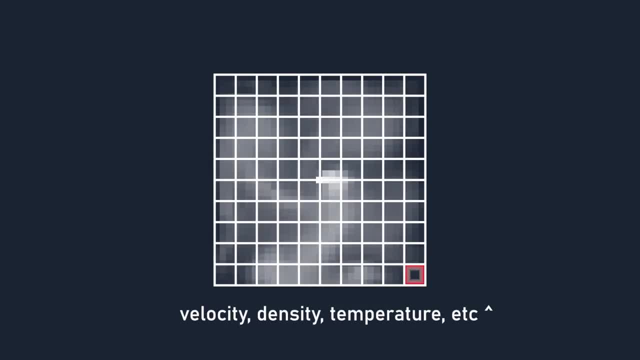 Now let's return to our 2D grid. Each grid square will have attached to it information about the fluid that is present in that square, the most important attribute of which is its velocity, how fast the fluid is moving and the direction that it's moving in, Of course. 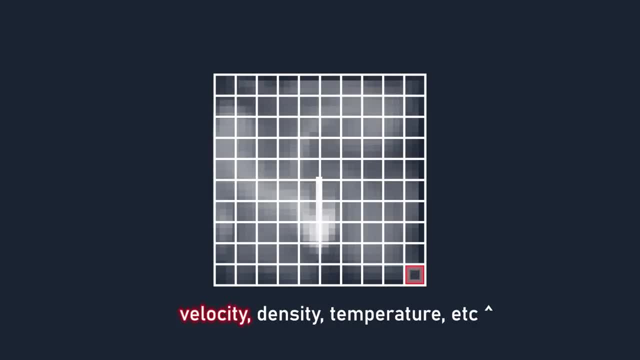 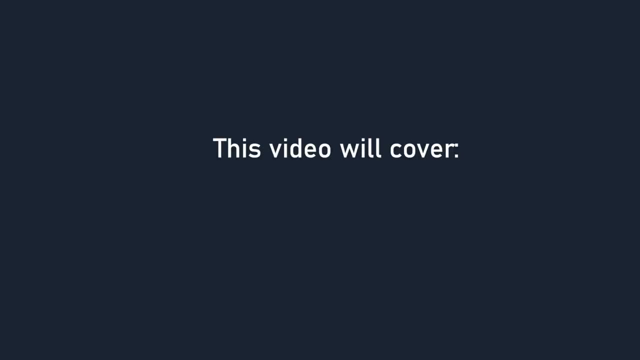 the most important feature of the fluid is arguably that it flows. Each grid, square can also have other attributes, such as density and temperature, but the way that all attributes distribute themselves around the simulation is very important. In this video, we'll cover the implementation of velocity and one other attribute, the density. 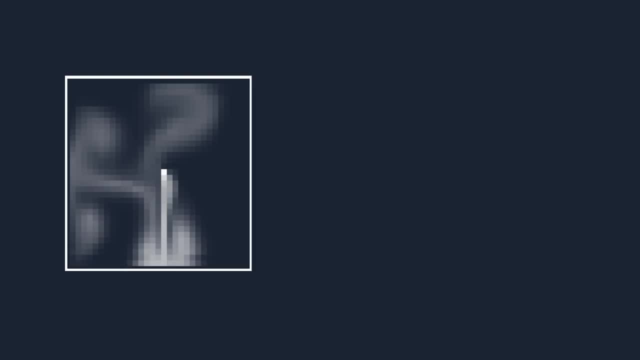 And the goal of the simulation is to take in a snapshot of all the attributes at a given time, then calculate how those attributes will change over many iterations and over many time steps. Of course, these attributes can also be continuously altered throughout the simulation as an input to be interacted with. 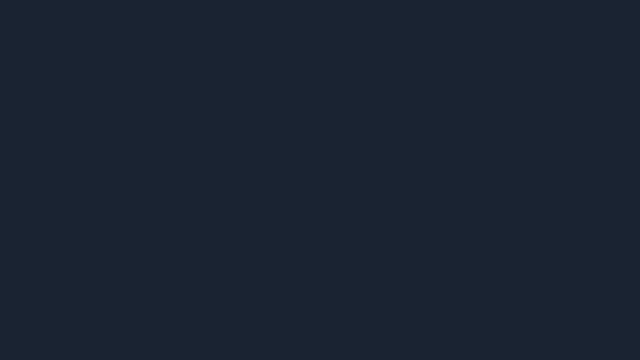 The first feature that we'll go through is actually not dependent on the velocities in the fluid. Diffusion is simply when attributes of each part of the fluid spread into the surrounding area, and the actual calculation involves making each square's value gradually become the average value of the squares surrounding it. Let's first consider diffusion of the 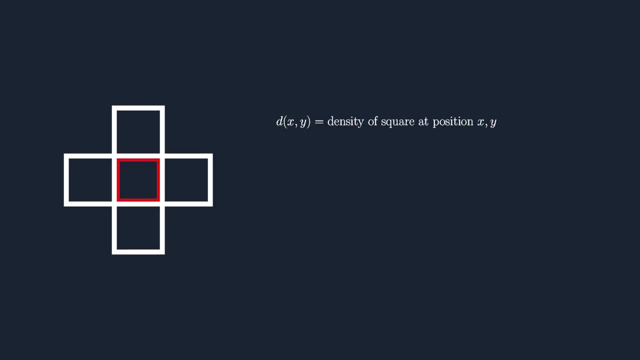 density. To see how this is done, let's let d equal the density of the square and s equal the average of the density of the square. Let's first consider diffusion of the density of the surrounding squares and k equal the amount by which we are changing the value. This amount will vary. 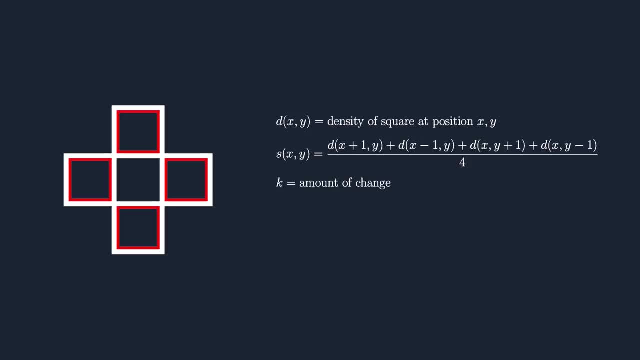 due to factors such as the time step and the viscosity of the fluid. Since we're trying to get the next iteration's densities from the current densities, let's use subscript c to represent that the value is from the current iteration and n to represent that it's from the next, Of course. 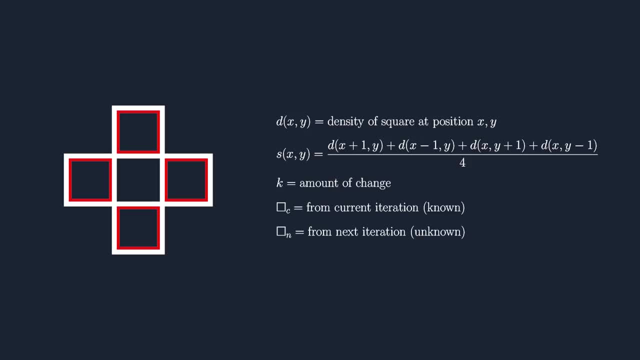 the current values are values that we already know, while the next values are values which we don't know And remember. we basically want to gradually make d become s. One way of gradually changing the values is to start at the current density. 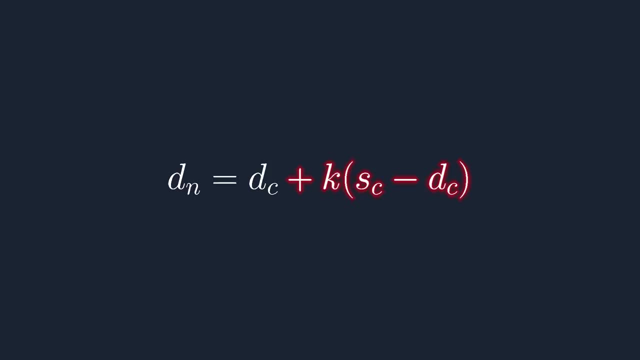 and then simply add on the difference between that and the surrounding average, multiplied by k, the amount. This is a linear interpolation, but that presents a problem When k is too large, specifically larger than one, we will actually overshoot the target value and go. 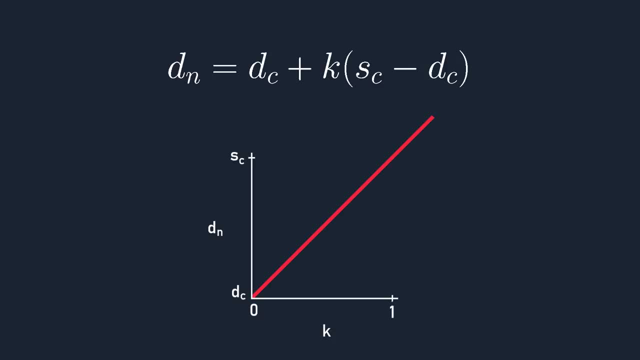 past it. This will result in unstable changes such as density values actually going negative and jumping up and down. Being able to look inside those changes will make the progress down unexpectedly. We can just cap k at 1 as well as that's unrealistic and limits. 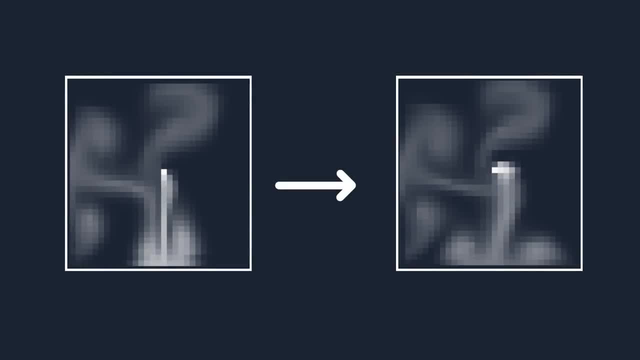 how fast the simulation can go. The solution is, instead of just using the current values to calculate the next values, we try to find the next values which, when rewinded back in time, result in the current values, Coming up with an equation to represent this. we. 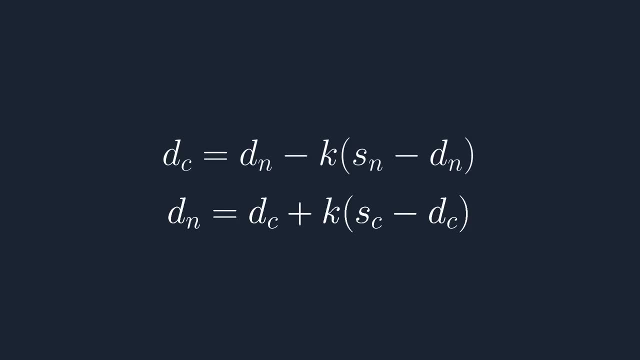 can see that it's very similar to the previous one, except the current and next are swapped and it's minus instead of plus. Rearranging this to make dn the subject, we can see that it's a hyperbolic relation and not a linear one. Now, no matter how big k is, we'll 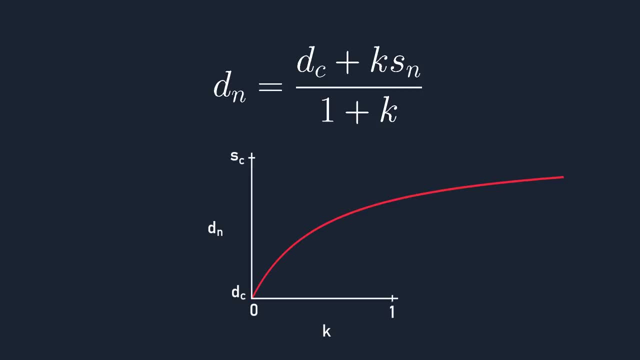 never overshoot the target value, but only converge to it. This is a stable way of interpolating, but it presents another problem. We need to know the next surrounding values for the calculation, which we obviously don't know yet. Let's expand out the s-value into what it really. 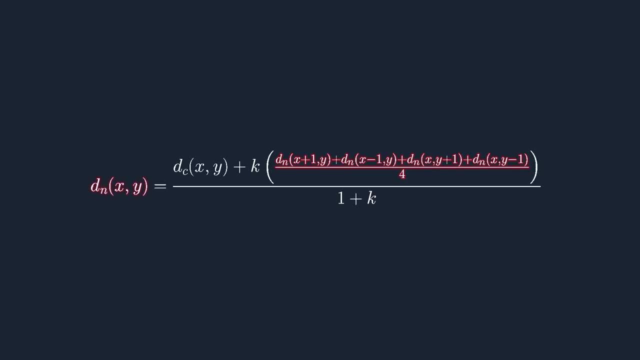 is the average of the surrounding d-values. Let's expand out the s-value into what it really is, the average of the surrounding d-values, Since there are many d-values and each d-values expression contains the other d-values. this is essentially a system of simultaneous equations. Now we humans can solve simultaneous equations. 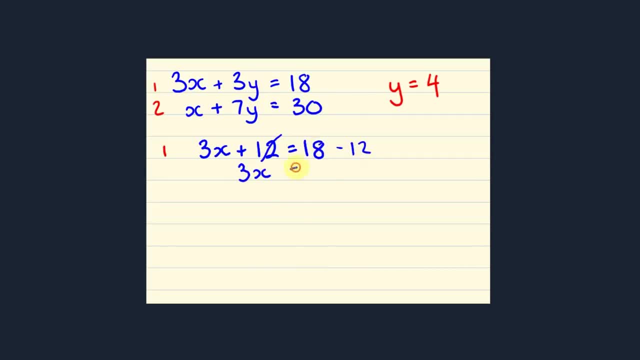 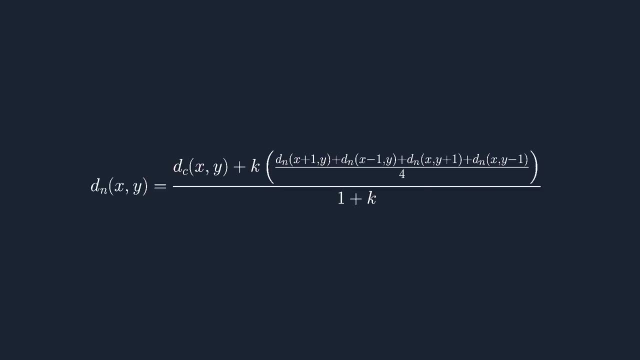 using different steps and coming up with different procedures depending what the system of equations is exactly, but we need the computer to be able to handle any system of equations, no matter what the values are, using the same procedure every time. Hence, we need to use 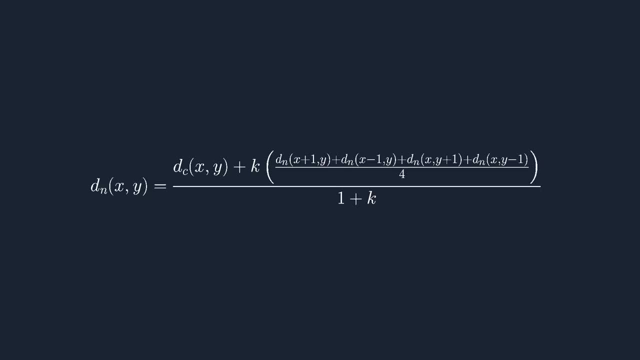 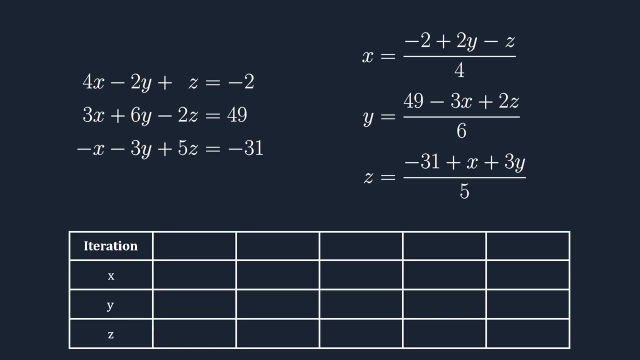 an iterative solver to approximate what the solutions are And remember the solutions are the dn values. The iterative solver we'll be using is called the Gauss-Seidel method. Basically, for all the values that we don't know yet, we assign something random to them, like 0. Now we know the values, but they're just incorrect. But 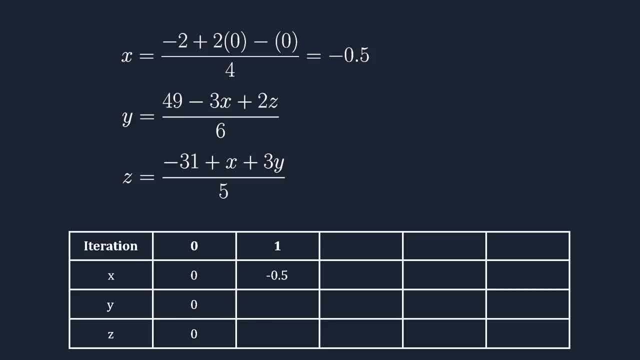 we can now start solving the equations using these values, updating the values with the new results we get from the equations. We repeat this process many times, each time using the newest updated values Very quickly. as we repeat it more and more times, the values we get converge to the true. 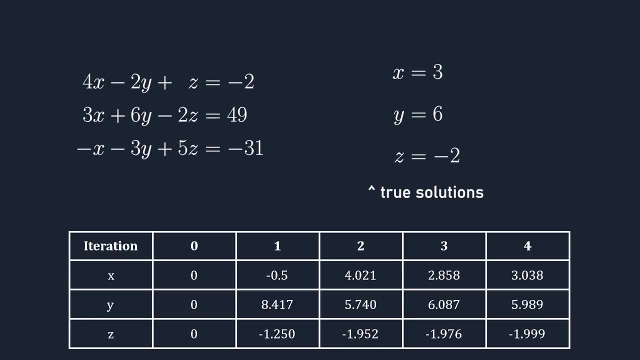 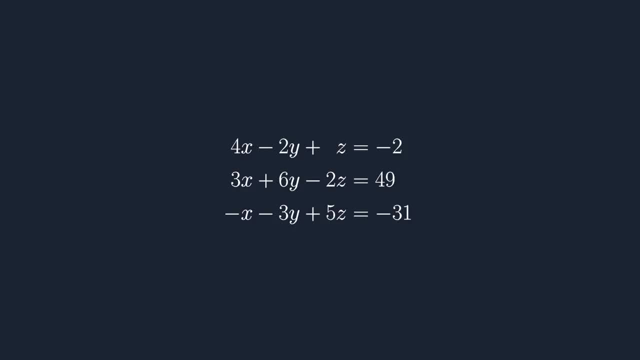 solutions for the system of equations. However, the Gauss-Seidel method does require a few conditions in order to work. Usually, the system of equations has to have a matrix that's strictly diagonally dominant, which means that the coefficients that lie on the diagonal have to have a magnitude that's larger. 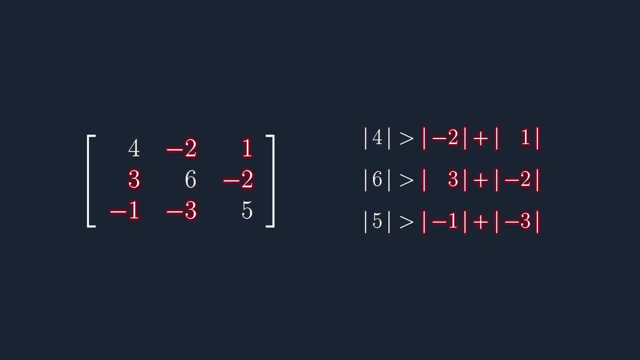 than the sub-diagonal. This ensures that in the solved equation for each variable, the variable coefficients don't add up to be more than the denominator, so the values we get are controlled and don't start blowing up. However, going back to our density equation, we can see that it already does satisfy this. 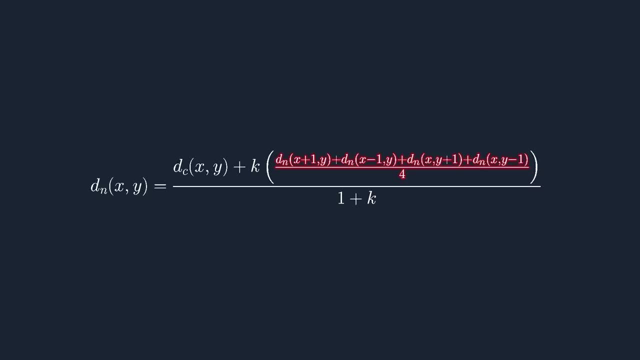 condition, since each of the coefficients is 1 over 4, and 4 of them added up, multiplied by k, will never be larger than the denominator of 1 plus k. So that's how we diffuse equations. Now let's look at some of the attributes in the fluid. We simply repeatedly solve an. 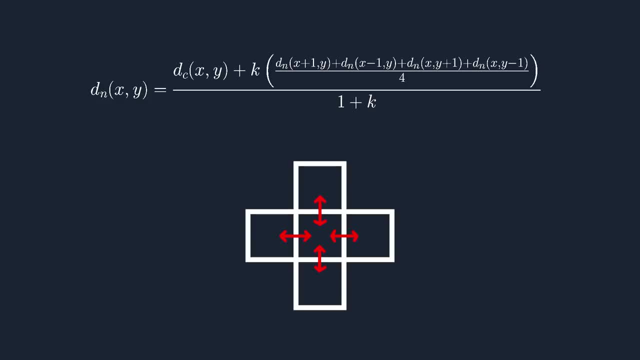 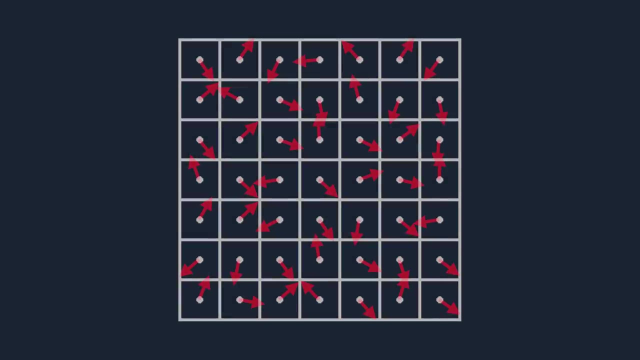 equation for each square, and their densities will converge to the diffuse densities that they are supposed to have. Advection is the movement of attributes through the fluid following its velocity. For the sake of consistency, we'll continue to consider the density attribute. This is a relatively 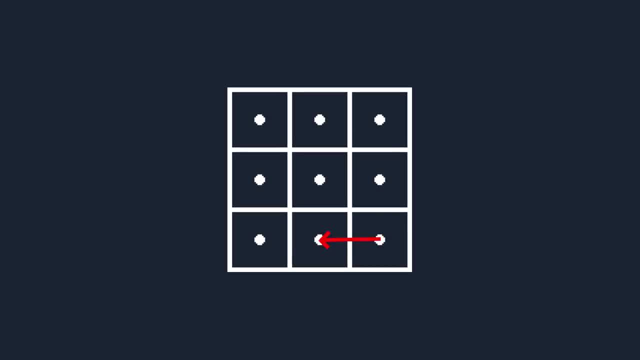 simple step. It would be even simpler if each square's velocity vector pointed exactly into the center of another square, because then we could simply move its density into the new square. However, the velocity vectors almost never point exactly into another square center, which means that 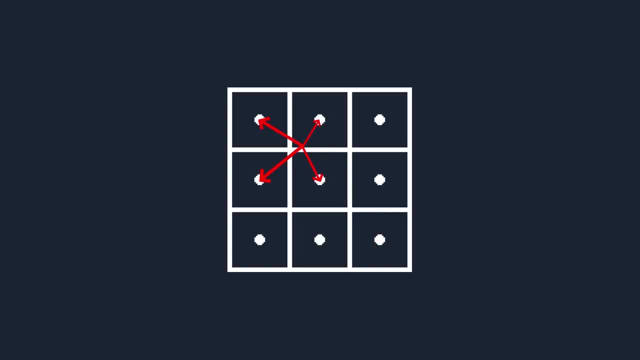 the density which moves following that vector will actually affect the four square centers surrounding the target spot. It's quite inconvenient to move density from their current positions into new positions and accurately distribute them into the surrounding squares, as there can be many vectors that move from one position to another and the density that moves from 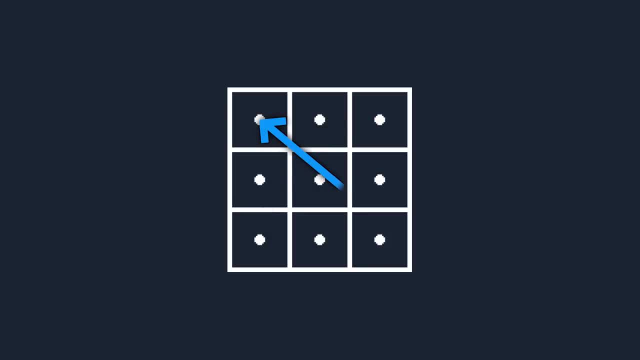 one position to the other, The density vector is pointing to the same spot. Hence we will once again trace backwards to find out where exactly its next density will come from. Where this resulting position is, we will linear interpolate between the four surrounding square centers' densities. 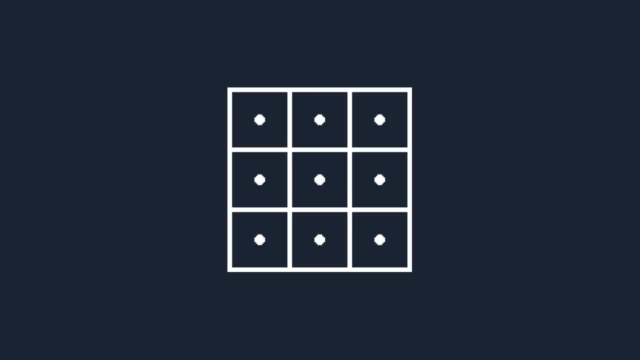 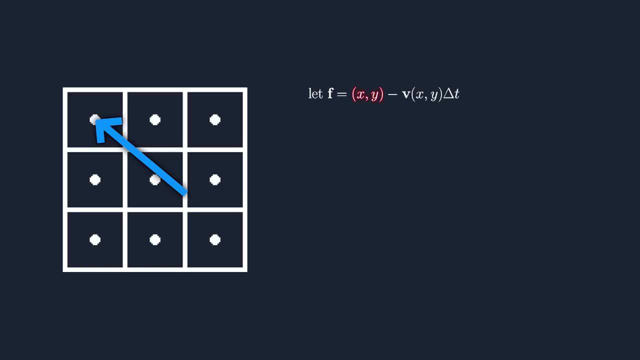 to find the target density. This way, each square only requires one calculation To find the position where the next density value is coming from. we can simply get the position of the square and subtract its velocity from it, multiplied by the delta time. Then 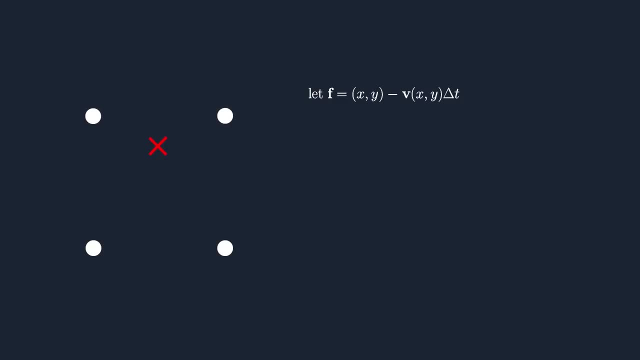 to find out what square centers surround this position, we can find the floor part of the coordinates, or in other words the integer part. To find the precise position in between those square centers, we can find the fract part or the fractional part, Then using 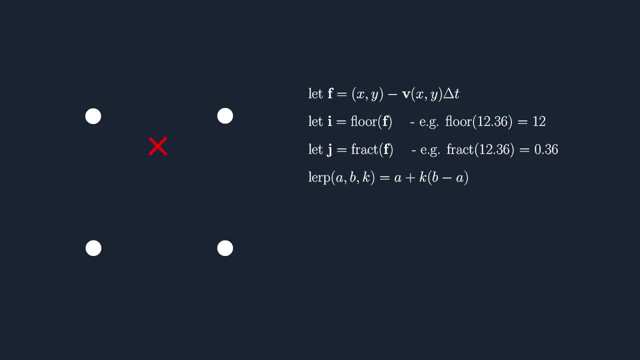 a linear interpolate function which looks like this: we can interpolate between the four surrounding square centers' density values by first individually interpolating between the two upper values and two lower values using the fractional x coordinates, then interpolating between those two results using the fractional y coordinates, And that 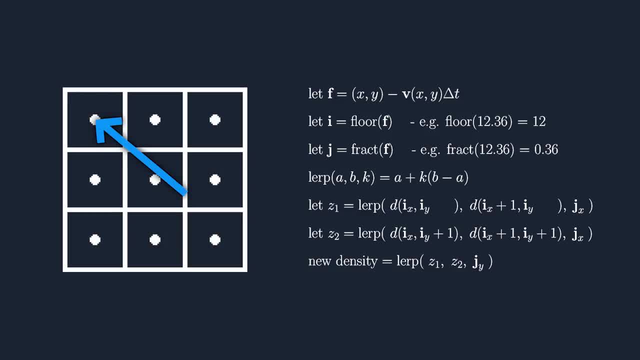 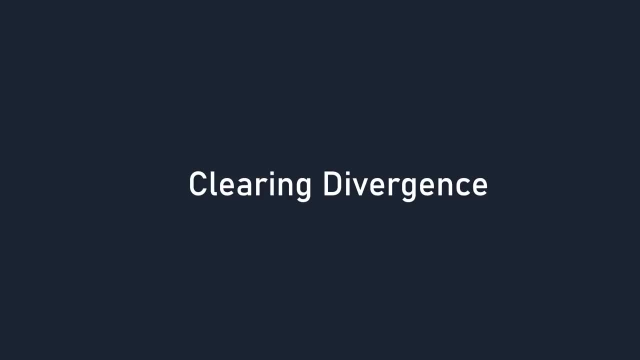 will give the new density value for the square in question. Clearing Divergence: I'd say this is the most complicated step in the whole video, so strap in. To understand this step, we must first understand the concepts of curl and divergence. Essentially, in a vector field, curl is when the vectors swirl. 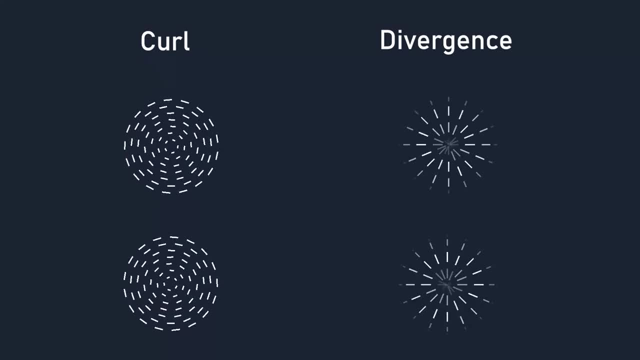 around and divergence is when the vector turns around and divergence is when the vector is either point away from each other or point towards each other. These two are properties universal to every vector field. Given any vector field, we can measure and find out. 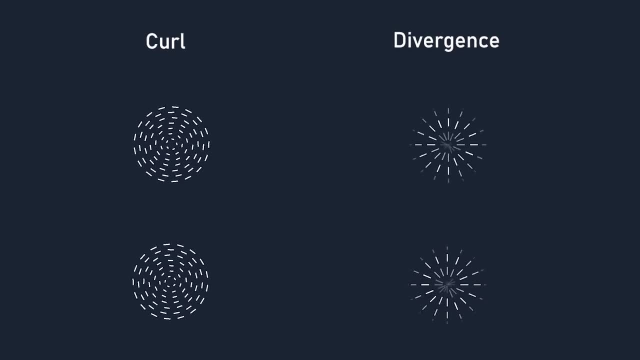 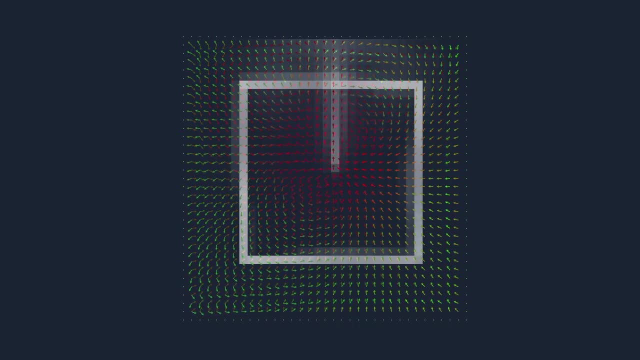 how much curl it has and how much divergence it has. Now let's think about a fluid. A fluid swirls around a lot, which means it has a lot of curl. However, if the fluid has divergence, that would mean that there'd have to be material. 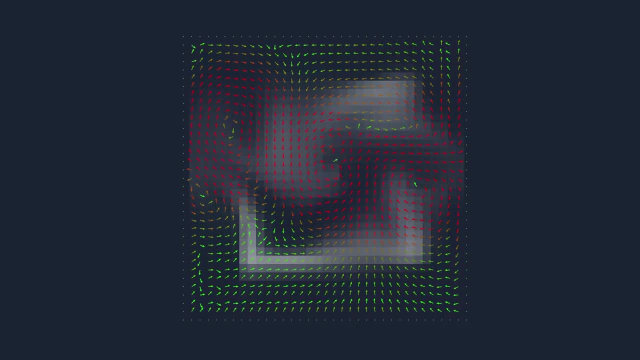 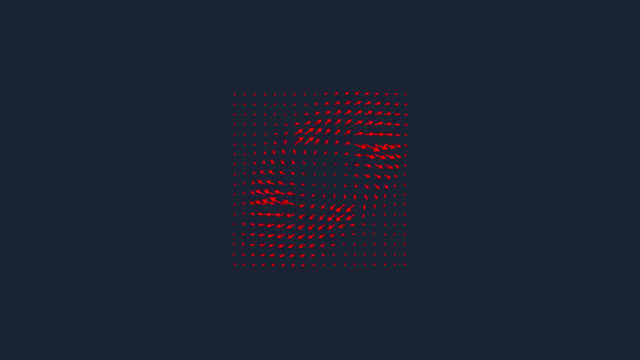 disappearing into nothing or material created out of nothing. Therefore, we want our fluid's velocity field to have curl but not divergence. However, after we do all that diffusion and advection to simulate the change in the fluid's velocity field, we actually end up with a velocity field which has both curl and divergence. 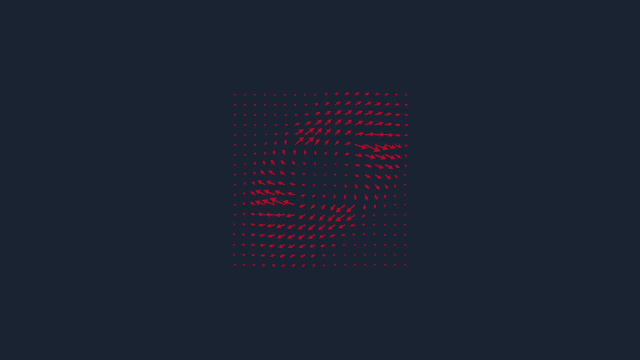 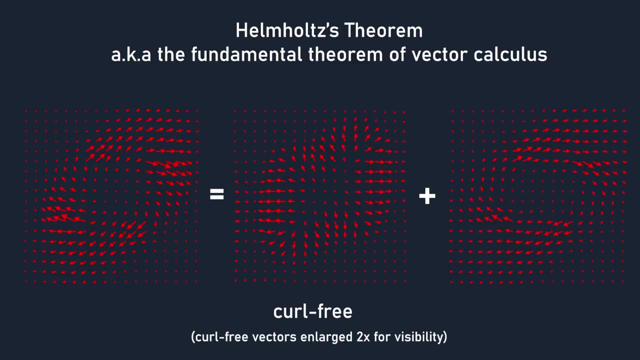 So we want to only extract out the divergence-free part. This is done through a process known as the Helmholtz decomposition. According to Helmholtz's theorem, also known as the fundamental theorem of vector calculus, Curl-free fields can be expressed as the sum of two vector fields, one which is free. 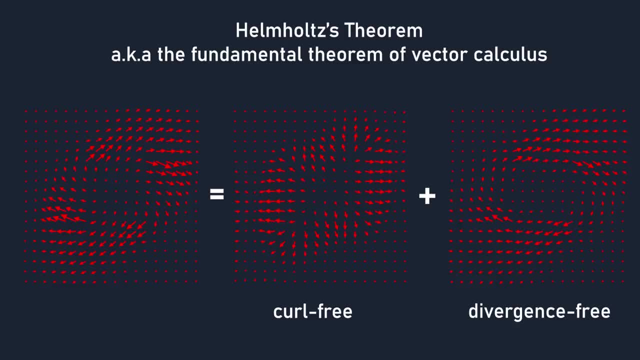 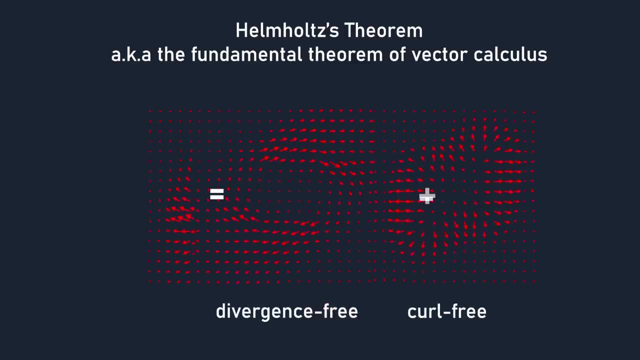 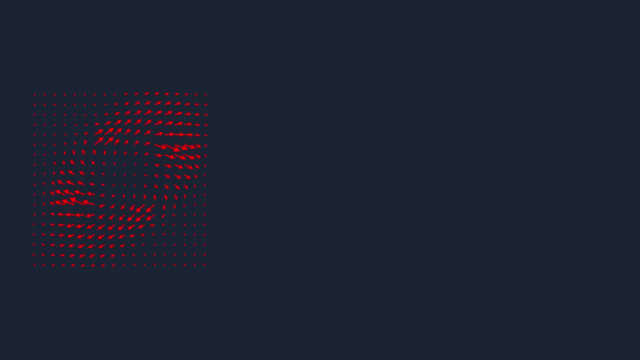 of curl and one which is free of divergence. There's no direct way to compute the divergence-free part, so our goal is to compute the curl-free part, then subtract that from the original velocity field to get the divergence-free part. First, let's calculate the divergence at each position in the field using this equation: 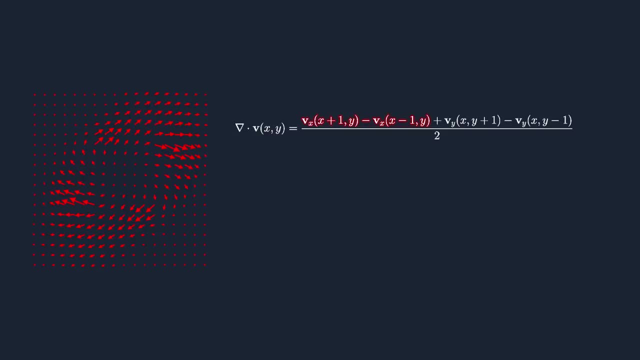 It involves a difference in x velocities across two horizontal squares plus a difference in y velocities across two vertical squares divided by the distance between those squares, which is 2.. To quickly visualize this, just on one axis we can see that if the larger position has 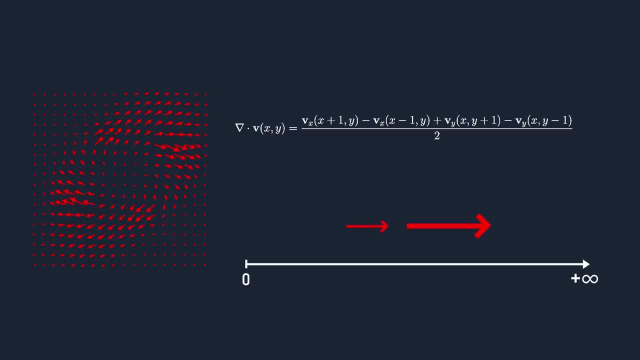 the larger velocity and the smaller position has the smaller velocity. there's more stuff flowing out than flowing in, and the divergence is positive. Vice versa, there's more stuff flowing in than out and the divergence is negative. After finding the divergence at: